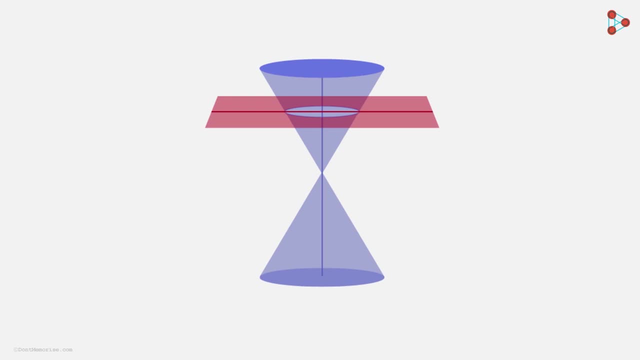 One way could be horizontally. Let's see, Let's see, Let's see. If a plane intersects the cone horizontally, that is, at 90 degrees to this axis, we get a circle. Yes, this shape here is that of a circle. 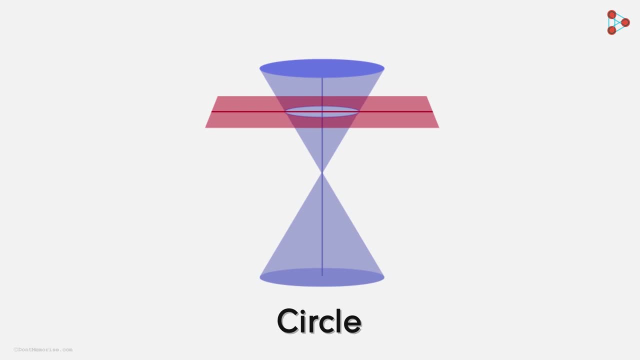 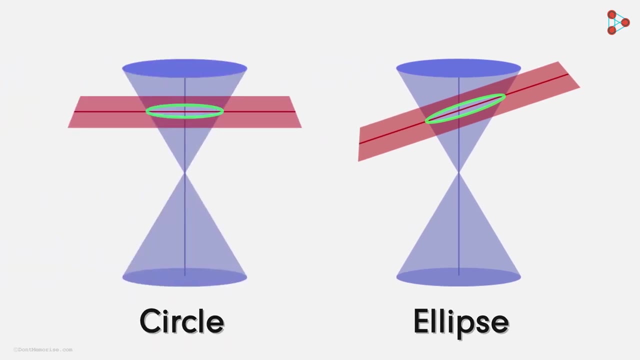 How else can this plane intersect this shape? What if we tilt this plane like this? We get an ellipse. If horizontal, then a circle, and if tilted a bit, then an ellipse. Let's continue tilting it a bit more. If we tilt it even more, 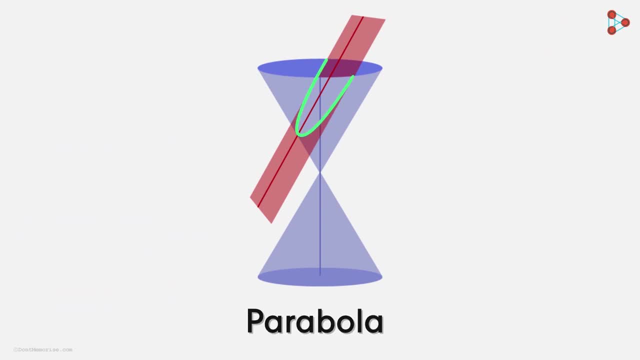 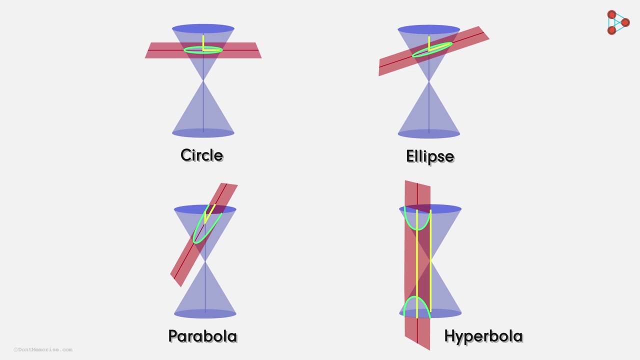 If we tilt it even more, like this, we get a parabola. And finally, if we tilt the plane like this, we get a hyperbola. So what can we conclude here? Depending on the angle at which the plane intersects the cone, we get different curves. 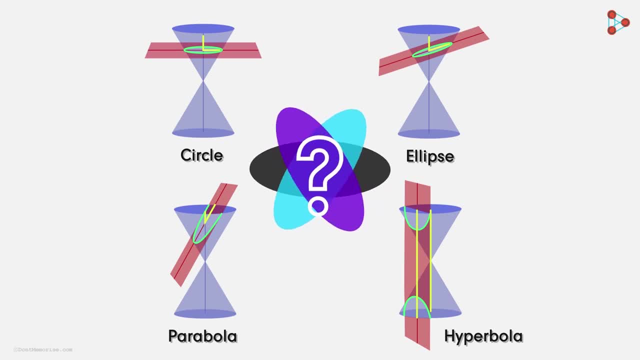 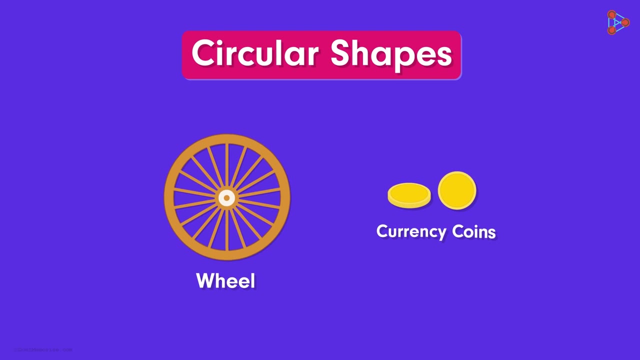 But why are we studying these shapes or curves? Because we see these shapes in our daily life, constantly, in some form or the other. Let's have a look at each curve individually. Most of us know about circular shapes. From wheels to currency coins, we can see many objects having the shape of a circle. 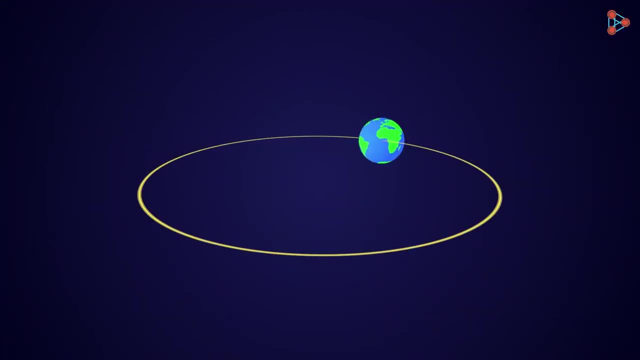 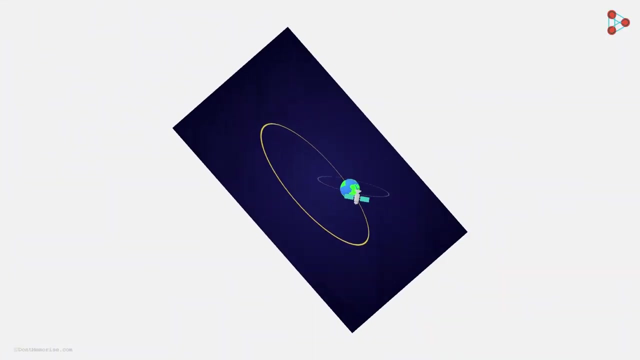 We saw that the earth revolves in an orbit which is an ellipse, And many satellites that are launched in space also move in an elliptical path. So just study the laws of the universe. Understanding the ellipse is important. Now can you tell me the shape of a satellite? 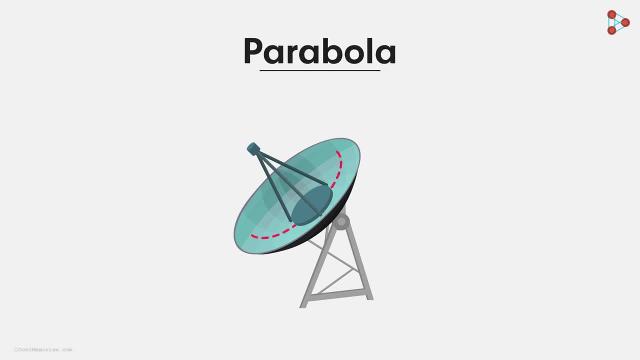 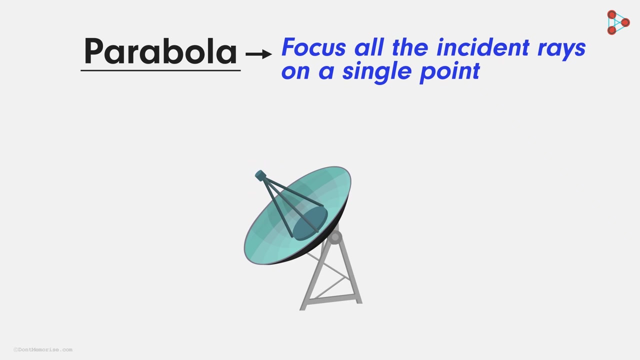 This curve is a parabola, So why do you think the satellite dish is parabolic in shape? Parabola has a property to focus all the incident rays on a single point. So if we keep a receiver at this point, all the reflected rays are focused here at this. 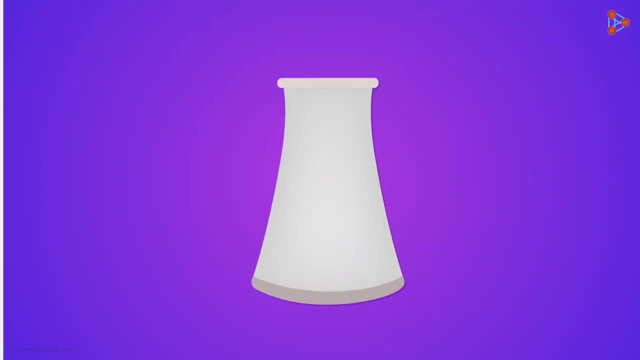 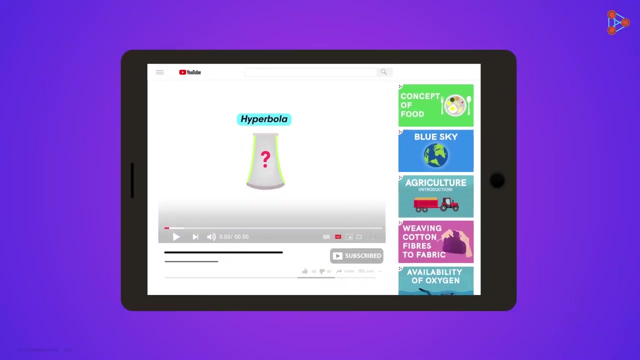 point Now. can you tell me the shape of this furnace? This curve is a hyperbola. Can you tell us Why do these furnaces are shaped like this? Tell us your answers in the comment section below. Do subscribe to our channel to watch more videos related to conics. We will launch them in the coming weeks.